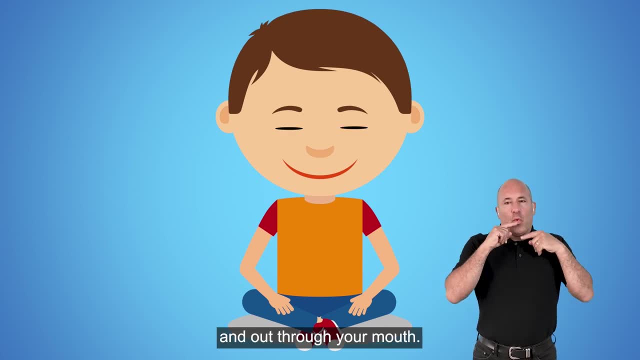 In through your nose and out through your mouth. In through your nose and out through your mouth. In through your nose and out through your mouth, Through your mouth. Good, After a few breaths you should start to feel nice and calm and relaxed. 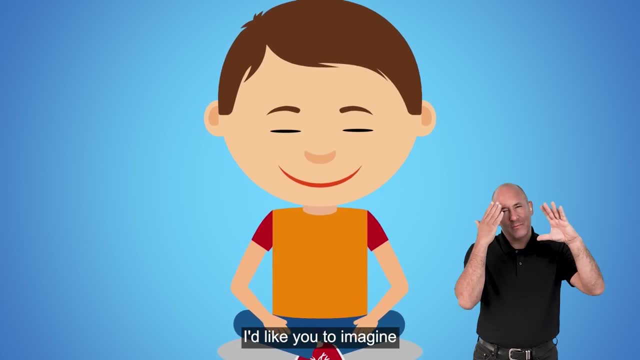 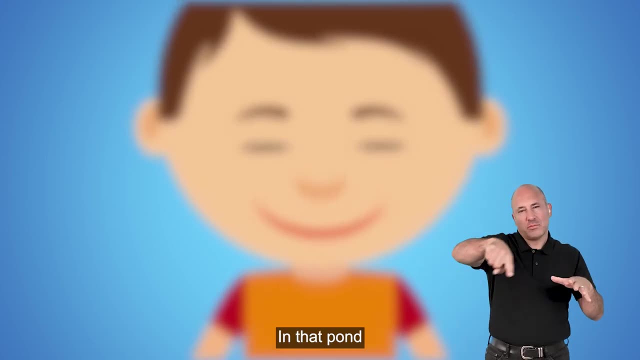 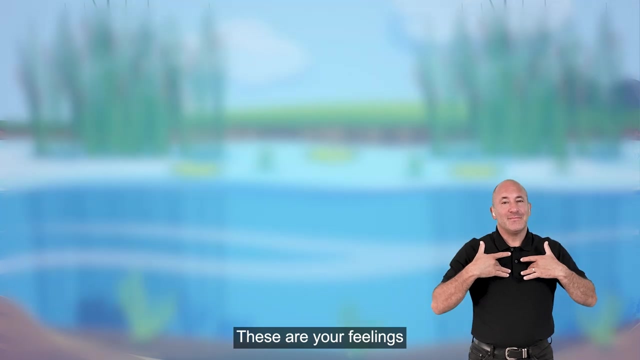 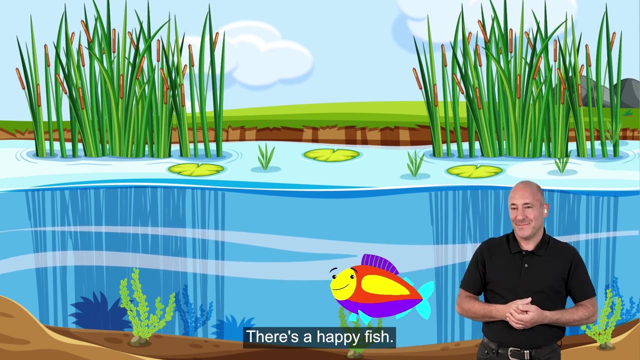 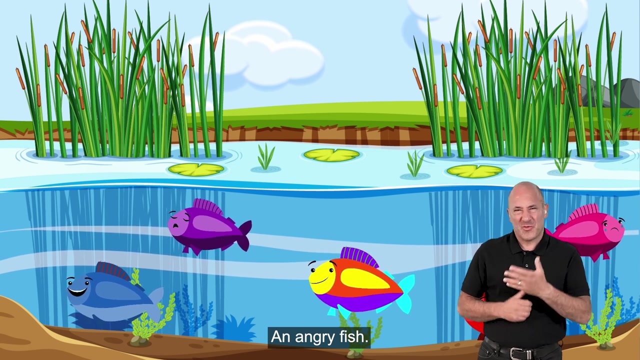 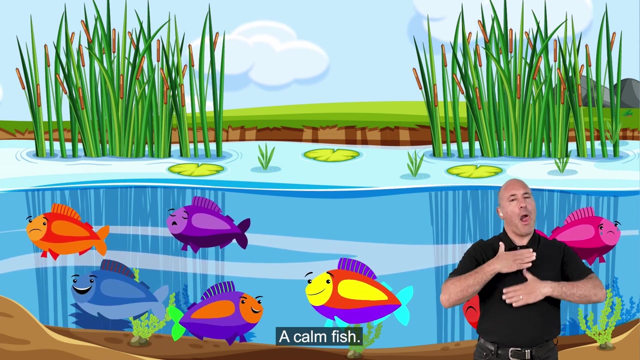 Now I'd like you to imagine that you and your mind is a big, lovely pond. In that pond are lots of different kinds of fish. These are your feelings All swimming around together. There's a happy fish, A sad fish, A sleepy fish, An excited fish, An angry fish, A worried fish, A playful fish, A calm fish. 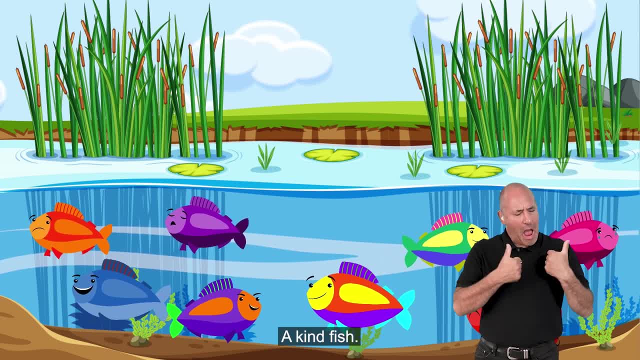 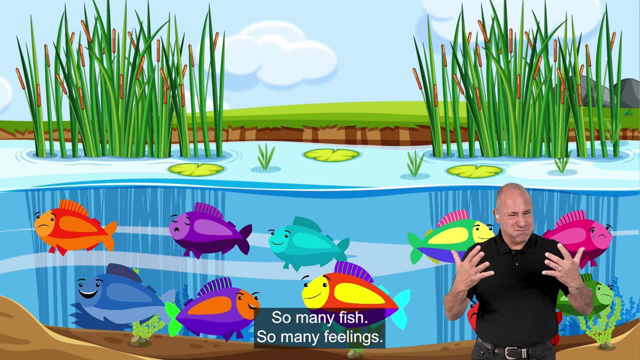 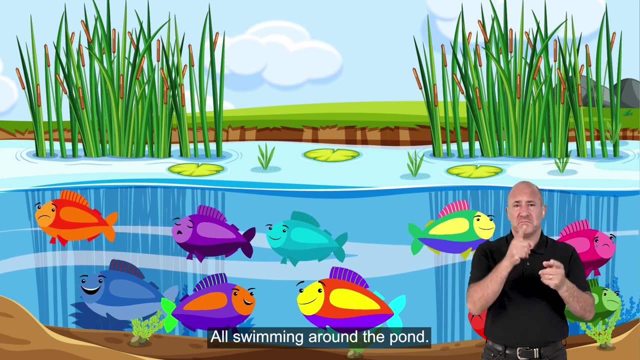 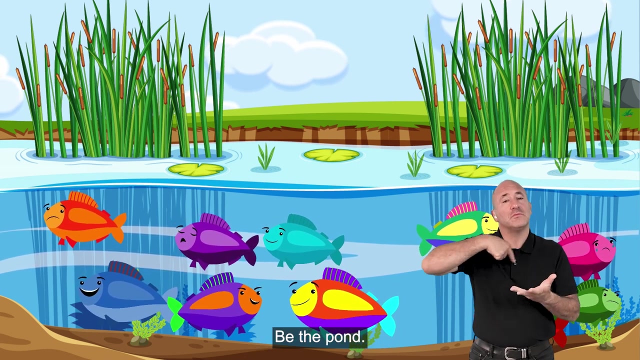 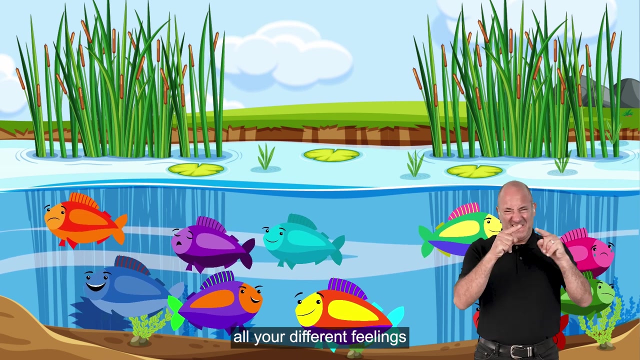 A kind fish, A selfish fish. So many fish, so many feelings, All swimming around the pond pond. Your job here is just to be the pond, Be the pond. It's wonderful being the pond because you can just watch all your different feelings just swimming by. All of them are. 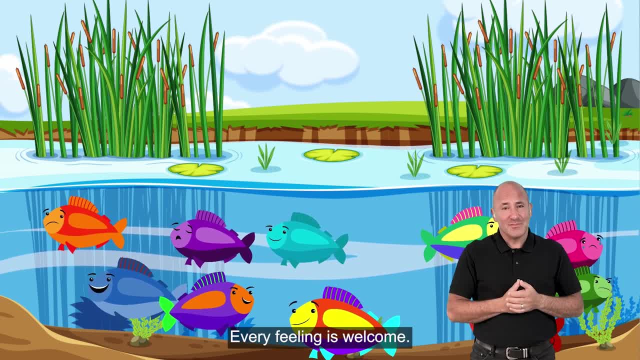 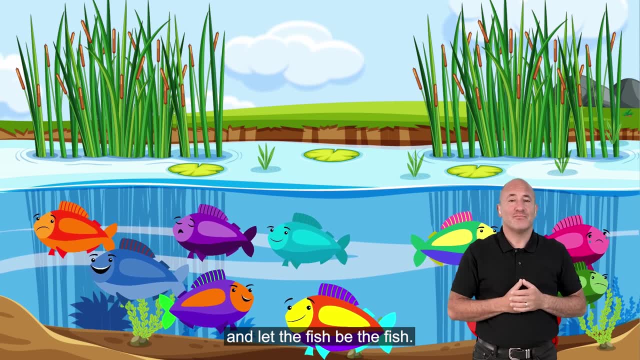 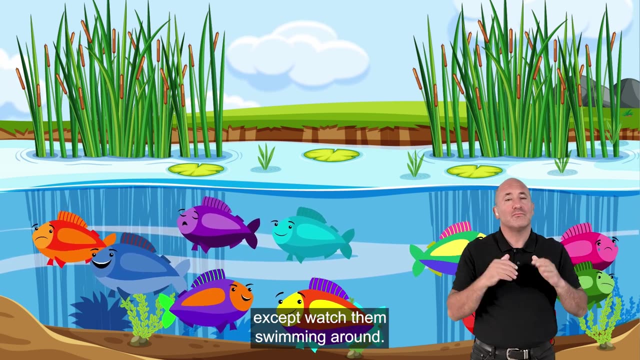 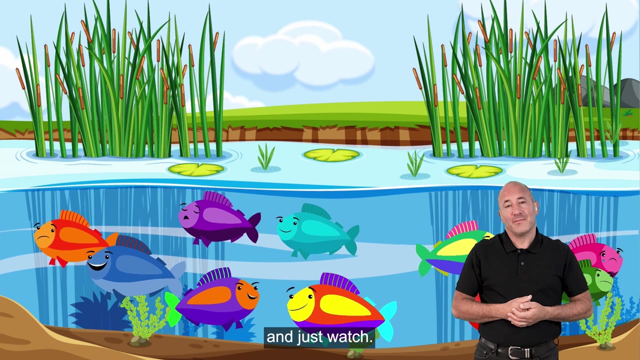 okay, Every feeling is welcome. You be the pond and let the fish be the fish. No need to do anything with those feelings except watch them swimming around. See if you can be the pond now and just watch, Seeing what kind of feelings you're feeling. 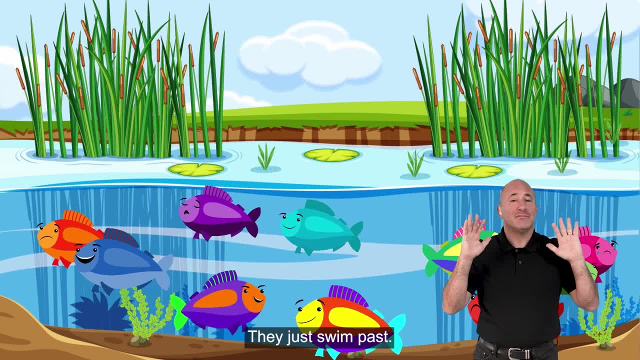 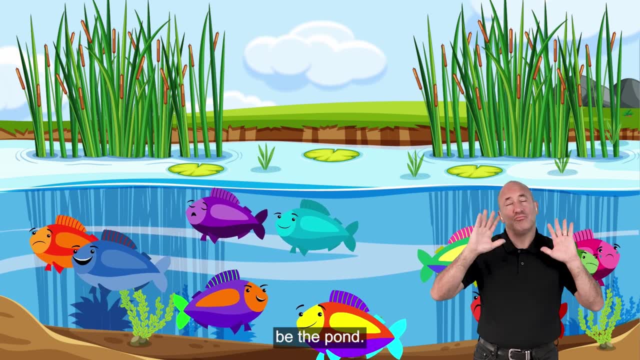 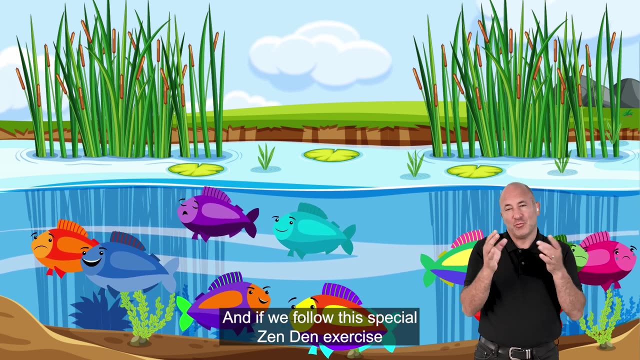 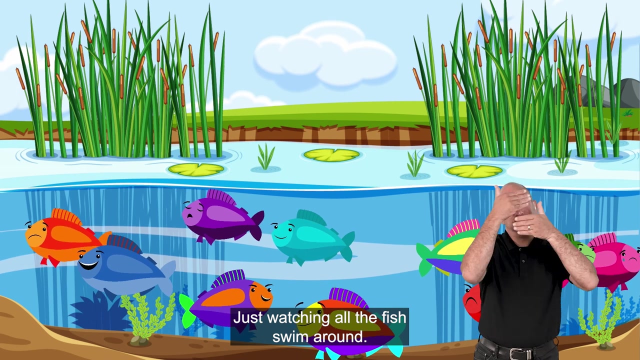 They just swim past and you can just watch them. Remember, be the pond, Just be the pond. And if we follow this special Zenden exercise, we are usually okay, just watching all the fish swim around, Except sometimes we don't want to be the pond, We don't want to be the